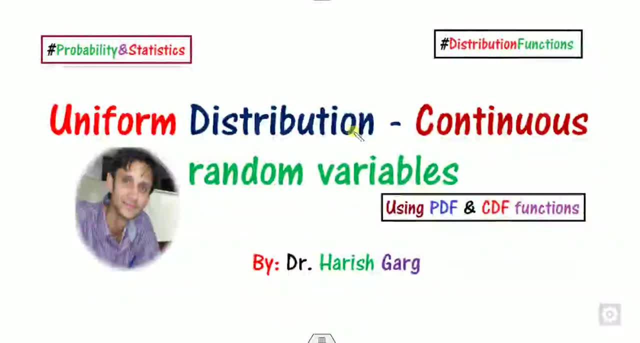 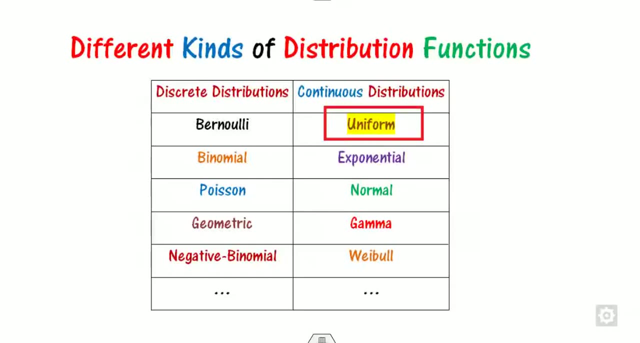 Hello everyone, Welcome to the next lecture on the distribution function. Today we will start with a series that is called as the continuous random variable and the corresponding distribution we will discuss here is uniform. So myself, Dr Garg, working in the School of Mathematics Thapar Institute. So what we have covered in the different kinds of the distribution function so far, So we have discussed all those here and which are available in my YouTube channel, is there. On the other hand, in this case, 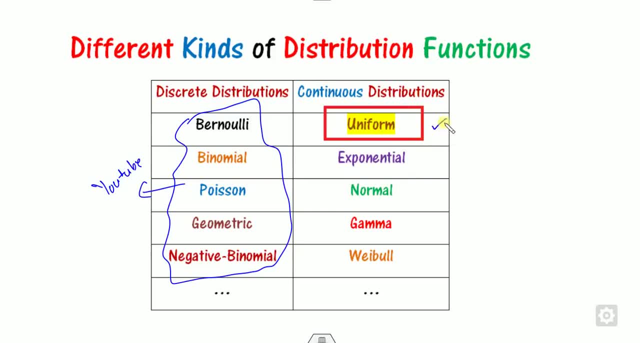 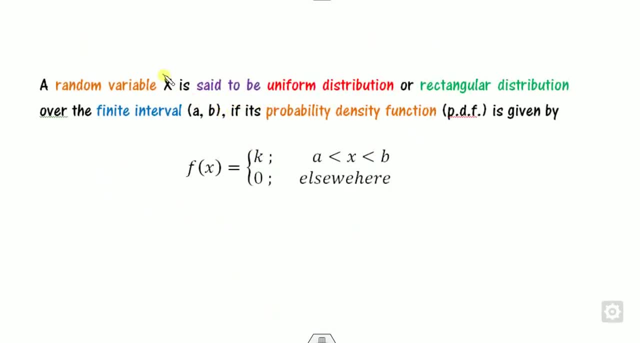 we will start with this continuous distribution and today we will discuss about the uniform and later on we will follow by this procedure. So what is the uniform distribution? Is there any random variable? x, which is said to be the uniform distribution- It is also called as the rectangular distribution, If its PDF function is defined like this way, that is, a constant from a to b, otherwise 0.. So now my main task is to find what is the value of the k so that it becomes the PDF. So there are the two. 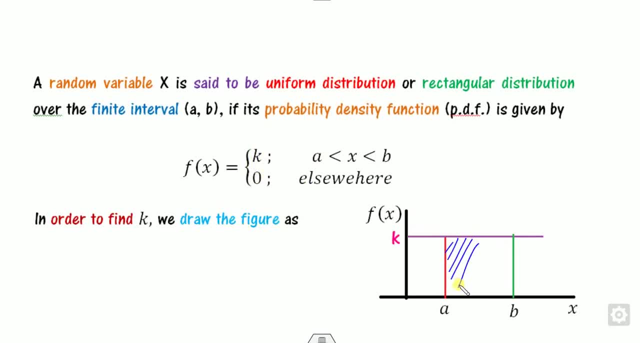 ways. First one you can draw simply graphically, So this is a portion. Look at that: whenever x lies between a to b, the function values remain the constant. So it is a rectangle. So, and since it is a probability, so the area of this is 1.. So how? and this is a rectangle, So what is the length of? 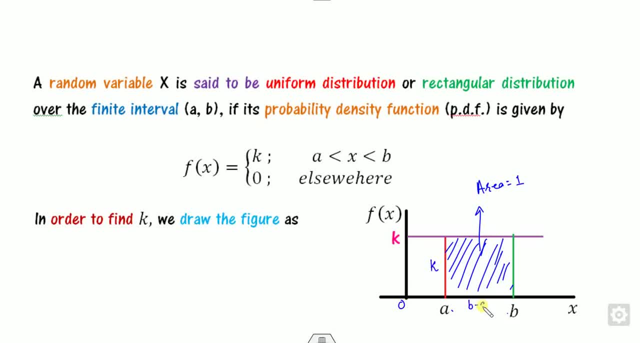 this is: This is my 0. So this is k and this is b minus a. So this is length into breadth, This is equal to 1.. So you can find k as 1 upon b minus a. This is the first method. Second method: you can use the definition of the PDF. 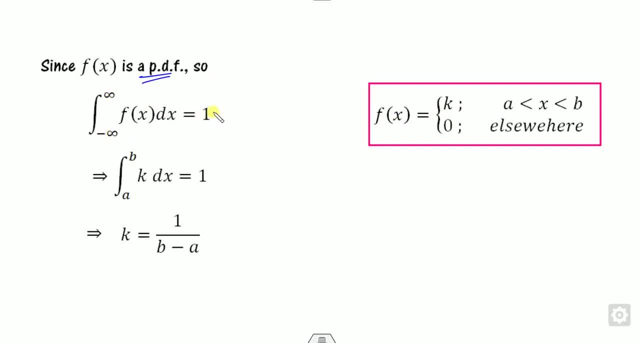 So, since this is my PDF, So the definition is: minus infinity to plus infinity is 1.. So I can discretize this from minus infinity to a, then a to b and then b to infinity, and the values of this and these are 0. So here, after solving, you will get again: k is 1 upon b minus a. So therefore, 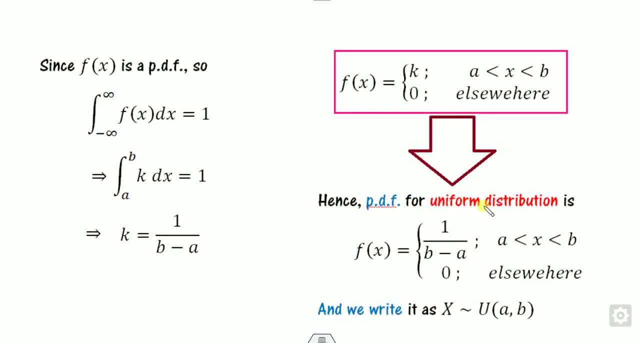 once we substitute the value of k here, you will get the PDF of the uniform distribution as this, And in statistics we denoted like this way: where capital X follows the, u is the uniform distribution, a and b are the lower and upper limits. So if you look at that, 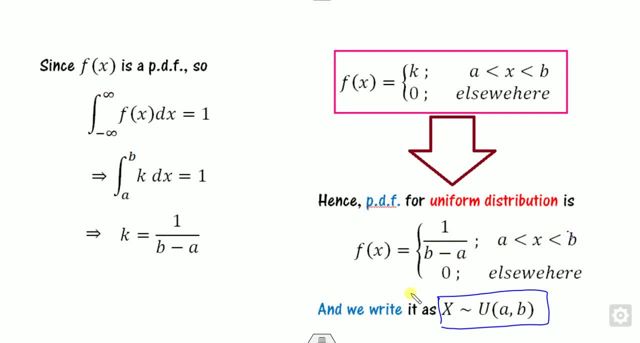 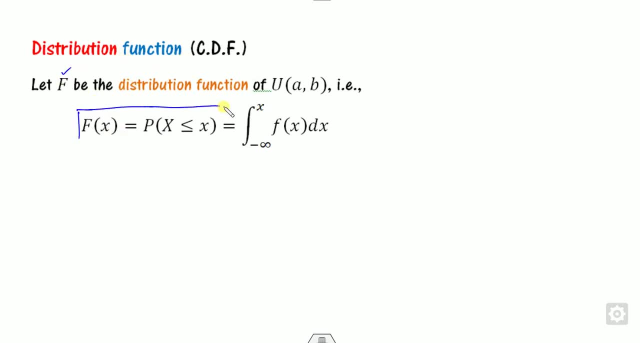 very carefully. this is 1 upon the range. b minus a is nothing but the range. Second concept we have used in here is the distribution function, which is denoted as a capital F, and its definition is here. So if you write this probability, so what is that? it's a lower limit is minus infinity. So you can. 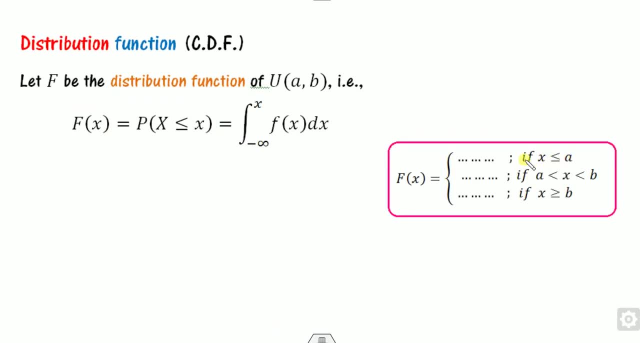 write it like this. So how you find this one? So look at that. my domain is x less than a, a to b and then so on. So my task is to find these three cases corresponding to them. So first case is when x is less than equal to a. So what is the meaning of that? It means, if I discretize this: 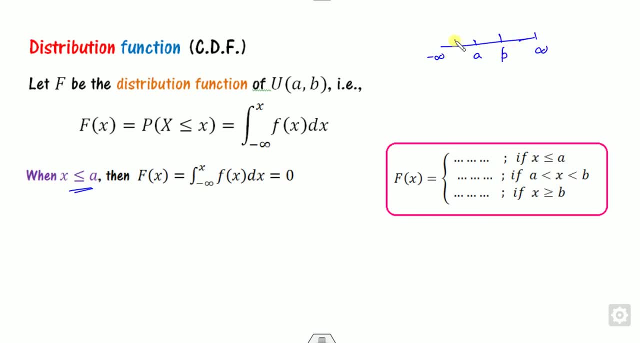 from here. So what is the meaning that we are case 1 here? So what is the value of the fx in that case? This is 0.. The value of the fx in between a and b is my k, or you can say this is: 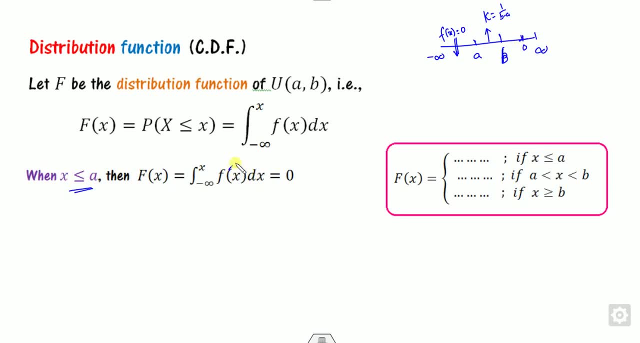 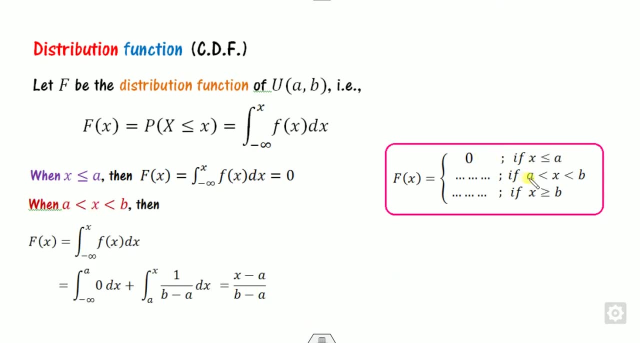 1 upon b minus a, and again this is 0. So look at, the value of the fx is 0. So the answer is 0. So this part is my 0.. Look at for the second case when x lies between a to b. So you have to discretize. 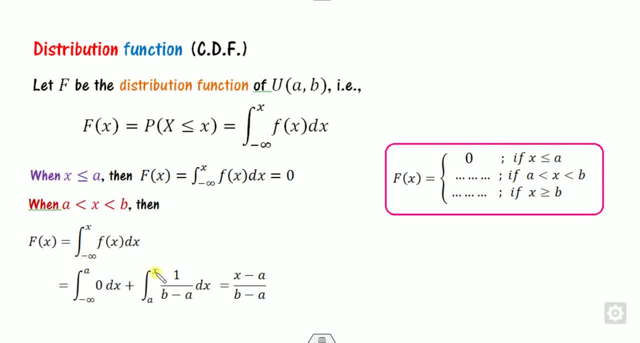 this from minus infinity to a and a to x. So what is the value of the minus infinity to a is 0 and from what is the value of the fx when lies between a to b, that is, 1 upon b minus a. So when you solve, 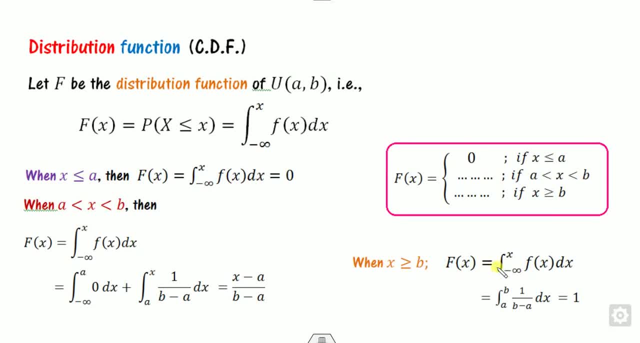 similarly, when you find the x is greater than equal to b. So how you find that you can break this from minus infinity to a, then a to b and then b to infinity. This value is 0. from a to b, This value is come to be 1.. This value is my 0. So the answer will be 1.. So hence this is my pdf, So you. 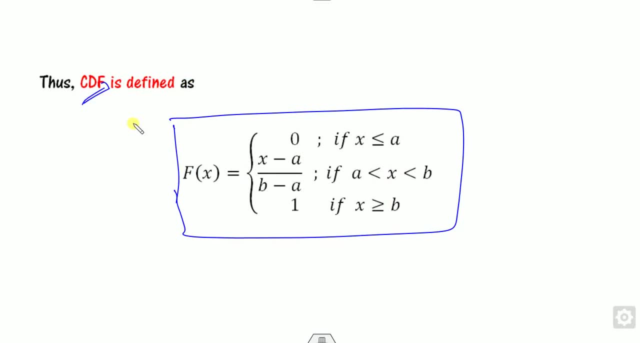 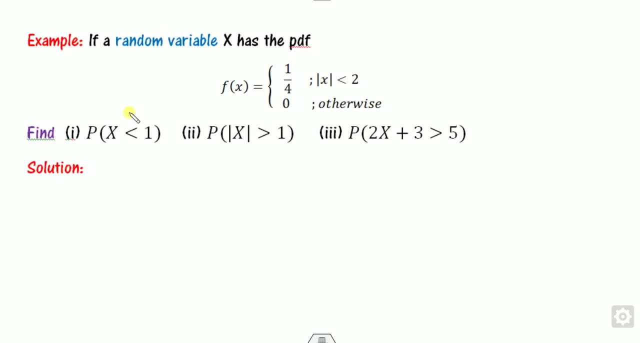 just remember this pdf, sorry cdf. So you just remember the cdf which will help to us to solve this problem. So let's do some one example corresponding to this pdf and cdf. Let us consider a random variable, x, which has some pdf is given to you. Then you have to find this probability, So what? 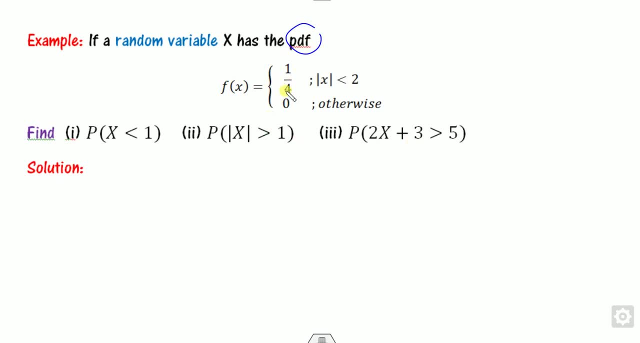 is given to you. that, firstly, is it. is it a uniform distribution function? It is not given here. But look at that. this is 1 by 4.. I can write this mod of x in terms of s and look at that, is it 1. 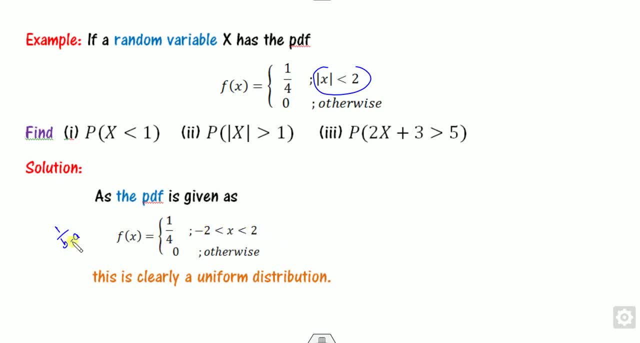 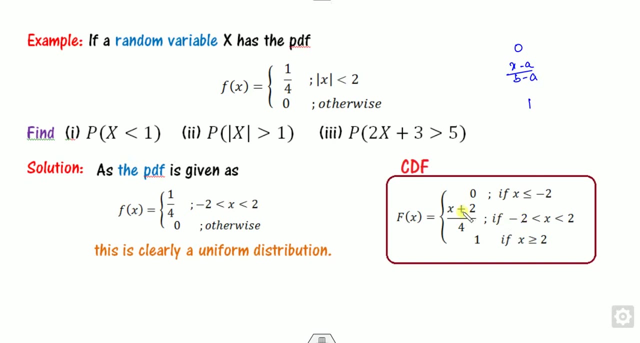 upon b minus a. Yes, because 2 and minus of 2 is there. So it means this is a uniform distribution. So if it is uniform distribution, then you can write this cdf also. What is the cdf is 0, x minus a upon b minus a and the 1.. So what is that? a is 2.. So x. 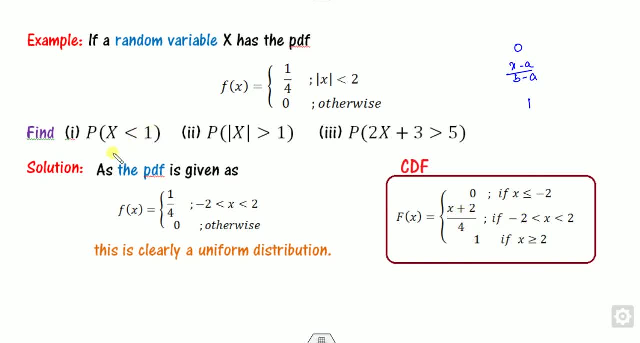 x plus 2 divided by 4, and so on. Now I can solve these three problems by using the pdf as well as the cdf, both- and you can solve it in in your examination, by any of the way, But I always prefer this because it give you answer within a 1.. 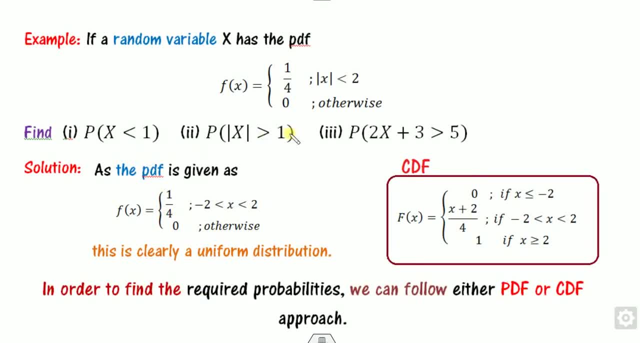 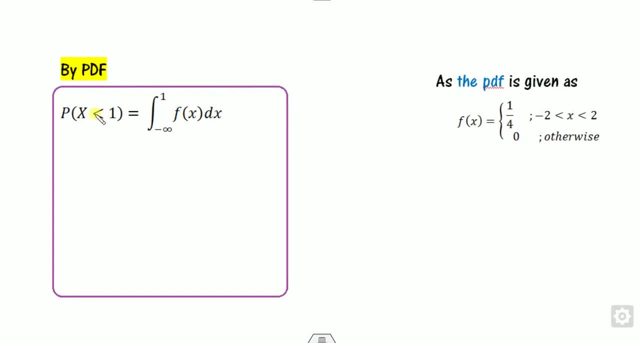 So 2 line maximum. So, in order to find the required probabilities, we can follow either the pdf or the cdf approach. So let us start with the first one. x is less than 1.. So what is the lower limit is minus infinity, So I can write this as minus infinity to 1 fx. Okay, So what is? 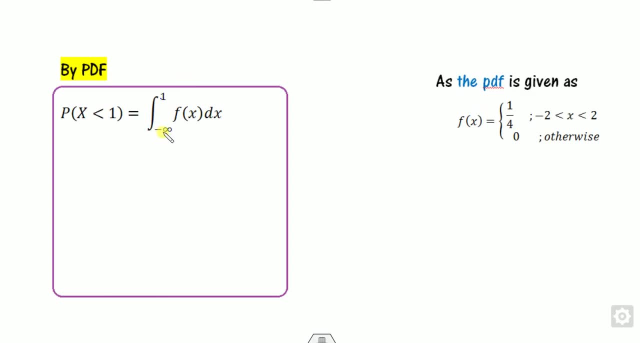 fx is given to be as a pdf. So this is my pdf approach. So now it is minus infinity to 1.. So, but the interval is from minus infinity minus 2 to 2.. So how you write that? I can decompose this. 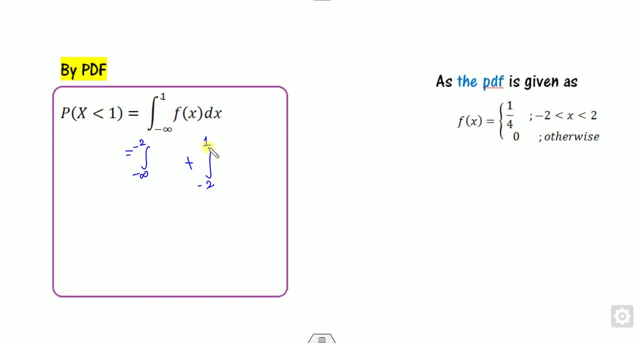 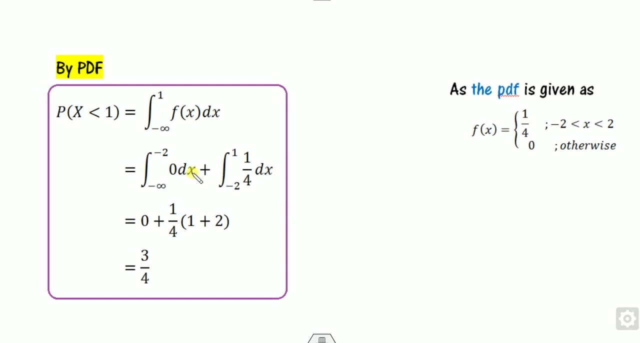 from minus 2 and then from minus 2 to plus 1. according to this, What is the value of the fx when x lies between minus infinity to minus 2.. This is lies otherwise. So this is values 0 and this value is my 1 by 4 into dx. So once you substitute here, look at that and how you solve. 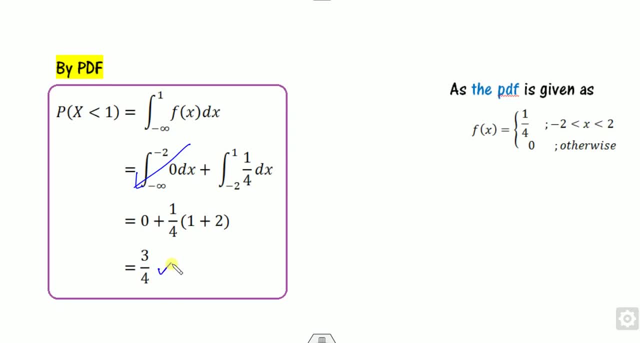 this value is 0. So 1 by 4 is outside upper minus lower, you will get 3 by 4.. So you can see that there is a three step answer is there? This is the first line, This is second line, This third line. 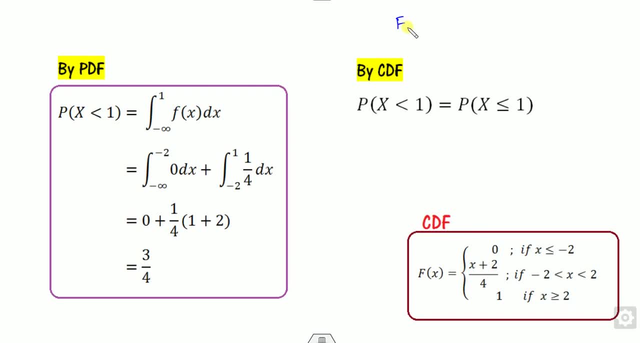 You can use the cdf always. remember that whenever you are trying to write the cdf, it means you have to find the capital F. So this is a capital F we have already given for the uniform distribution and the next task is, whatever the probability is given to you, You can write always in terms of the. 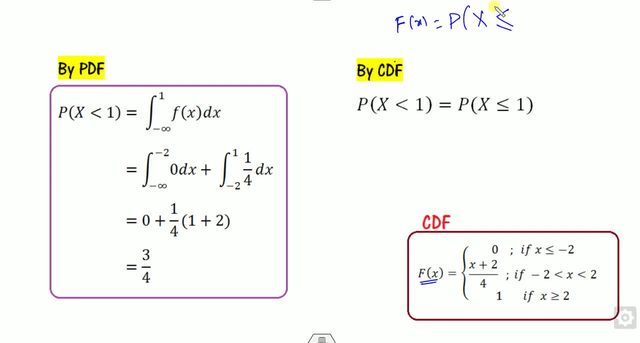 less than and equal to be. always remember you write less than or equal to now, since here its equality is not be there. but this, what is the domain, is my continuous random variable, and we have seen in our last lectures that for a continuous distribution function, that probability. 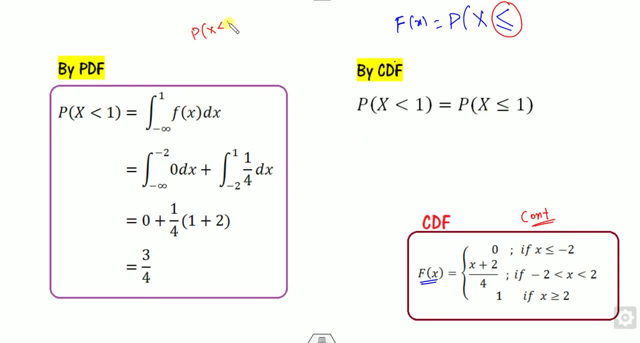 at a single point is 0.. What is the mean is, if I say probability at x is 2 and probability at s less than equal to 2, they all are same. So it means you can write is as a here. So what is that? What is the meaning of this? This can be. look at that whatever you have. 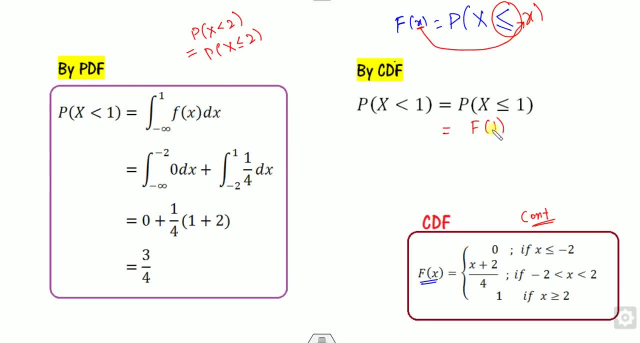 right here x, So the same x is here. So this is nothing but f of 1.. So where is the one lies? that one lies here, Okay, So you can substitute directly the value of here, So you will get as a 3 by 4 and you can see. 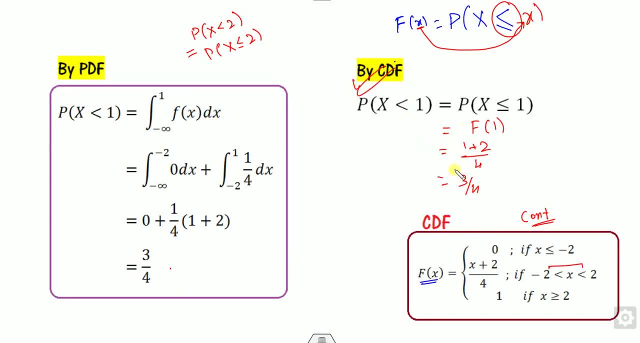 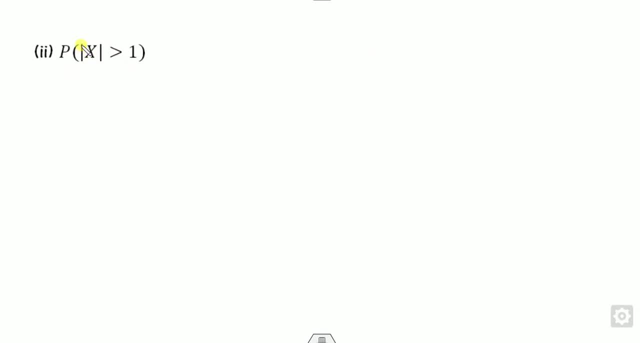 that both the answers are same. That's why I always prefer this cdf, which is given always in the one line answer. Look at the second part. is there? your task is to find this Now. since it's a modulus sign, you firstly convert into the single x, So I can write this as: 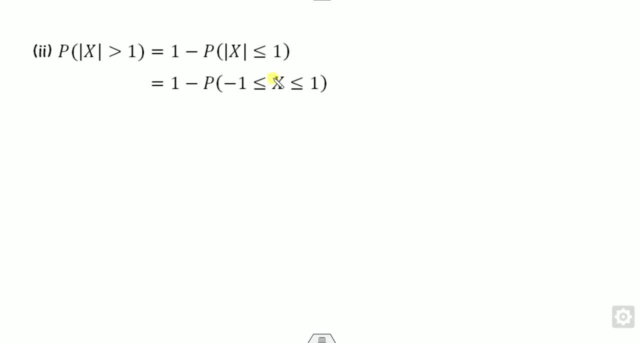 1 minus, and now it's a modulus. you can write here. Now again, there are the two approaches. one is using the PDF, second is using the cdf. So let's start with the PDF. This is my PDF function. How can I write: is this is one? this is PDF means that is integration. 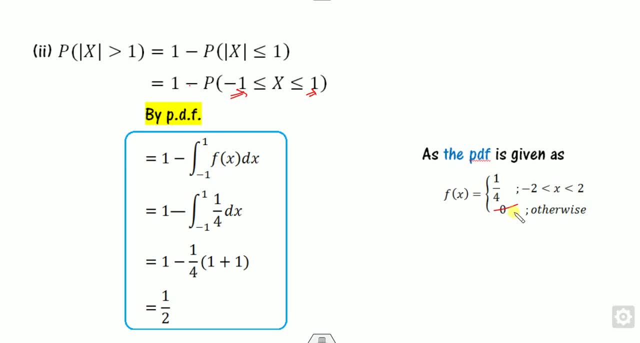 from lower limit to the upper limit minus 1 to 1.. So is minus 1 to plus 1 lies in this? yes, then there is no need to separate them, So you can substitute. what is the value of the fx when x lies between minus 1 to 1, 1 by 4.. So after solving, you will get 1 by 2.. 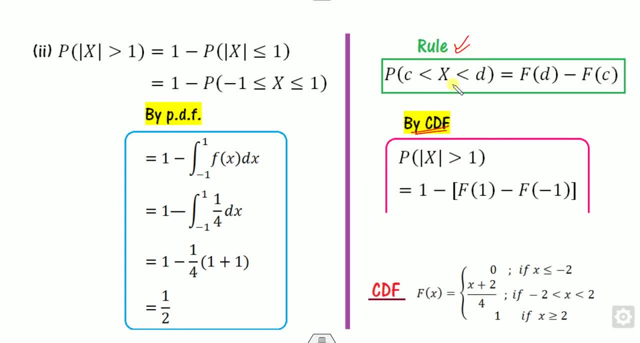 On the other hand, if you solve this with the help of the cdf- always remember that- we know that whenever the probability lies between minus 1 to 1, you will get 1 by 4.. So, after solving, you will get 1 by 2.. On the other hand, if you solve this with the help of the, 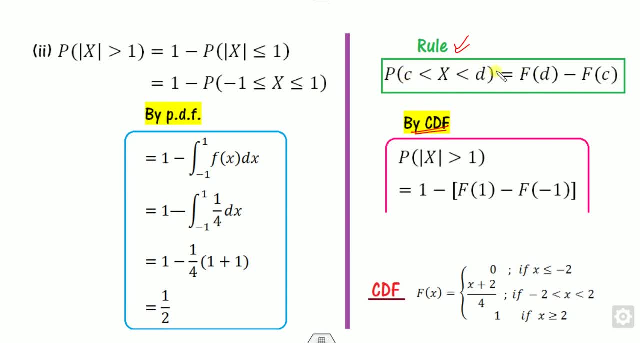 fx when x lies between the lower and upper, how you can write in terms of the cdf is f of the upper limit minus f of the lower limit. So look at that. we want to calculate this. So this is written as here. So how you write this as in terms of the cdf is 1 minus upper. 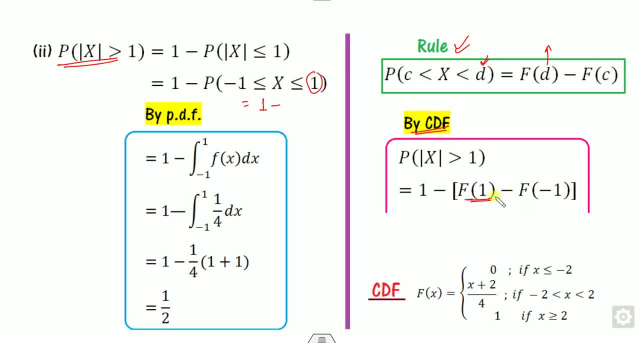 is 1 minus lower. Okay, So now, what is f of 1? this is a cdf. where is one? lies lies here, So you can substitute one. the value here, This is 3 by 4.. What is the? where is the minus? 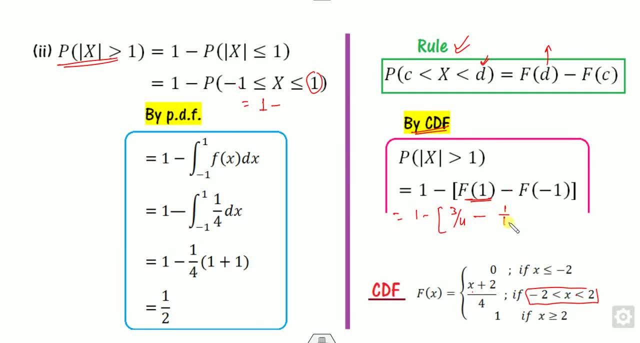 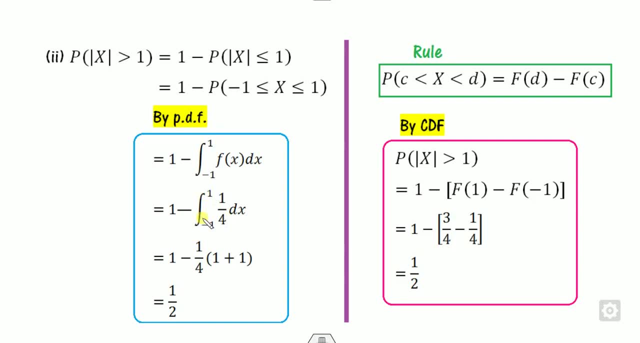 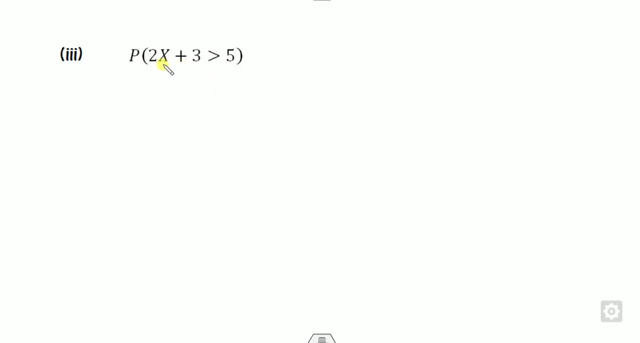 1 lies Again, So it will be my 1 by 4.. So this is the required answer. So look at that. always the three line answer. instead of finding an integration, You always find the answer with the help of the cdf better manner. Look at one more example. is there? Same question? is there? So look. 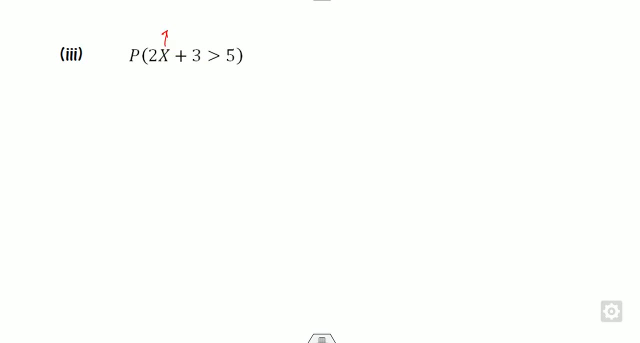 at that. So firstly, we have to simplify this. find the value of the x from here, So we can simplify this, as x is greater than 1.. So now by using the pdf rule, how you find this. This is the pdf. So this is greater than 1.. So 1 to infinity, But my domain is from minus infinity to 2.. 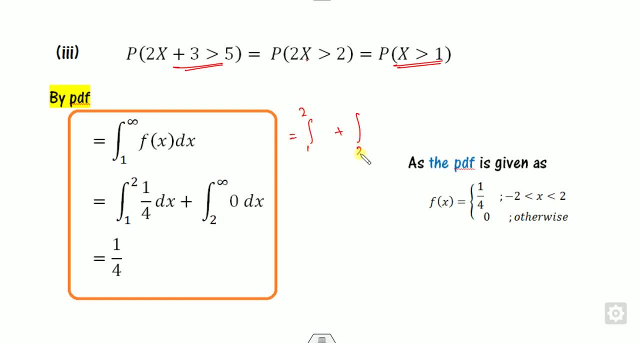 So how can I write x from 1 to 2 and then 2 to infinity? What is the value of the 2 to infinity is 0. So this is 0, and 1 to 2 is my 1 by 4. So this is 0. So you can write. 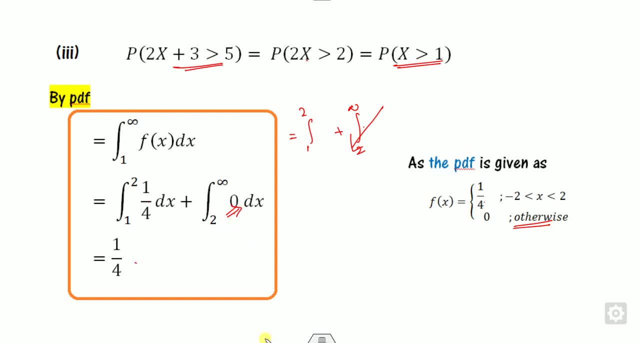 this as 1 by 4 is the answer. On the other hand, if you write this in terms of the cdf, My task is always I How I write that. My task is always to write in the less than equality form. So how you write this term. 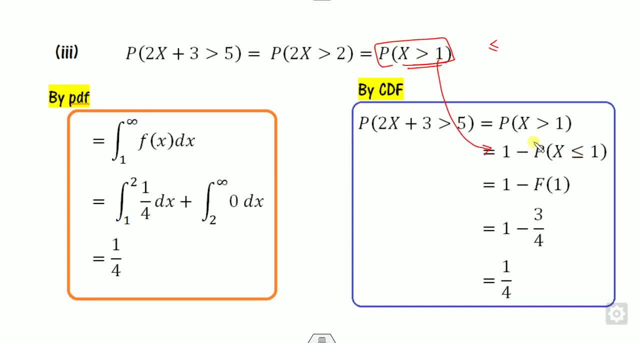 as a less than equality. So look at that. This is there. So what is that? This is nothing but my f of 1.. So I can substitute the 1 value as 3 by 4.. Look at that. answer remains same. 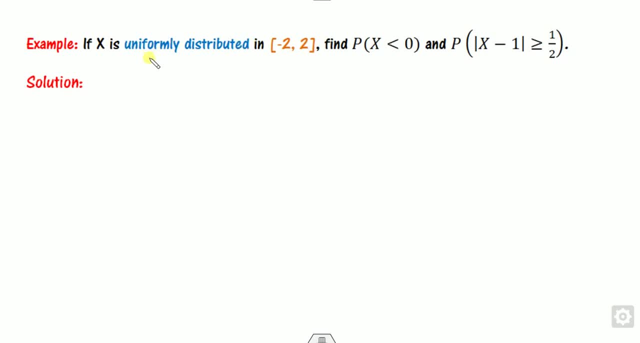 No problem, we will continue in the second example So it will be more clear. So let x be a uniform distribution over the domain this and you have to find this. So it is given that it's a uniform distribution. So how you define the pdf? 1 upon b minus 1.. So this: 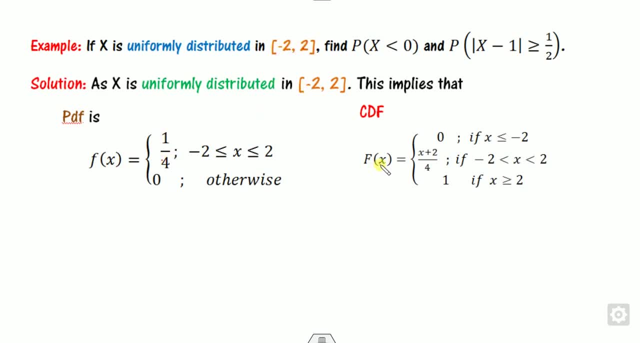 is 1 upon b minus a. So 1 upon b minus a is this? and what is the cdf is 0 x minus a by b upon a. So look at it Now. you have to define, you have to calculate this value. Firstly, 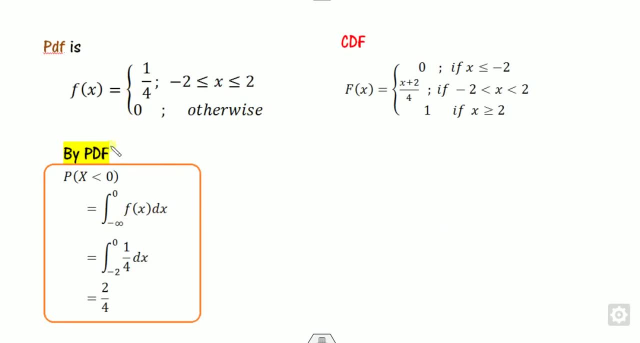 again, we apply the pdf and the cdf rule. If you apply this by pdf, how you solve this? minus infinity to 0. Is there need of the breaking? Yes, Okay, How you break them is from minus infinity to minus 2.. And then minus 2 to minus infinity, to minus infinity to minus 2.. So 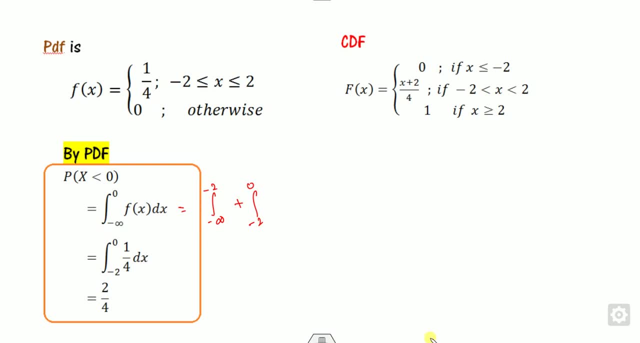 what is the value of this minus infinity to minus 2.. This value is my 0. And what is the value of minus infinity? This is 1 by 4 of dx. So when we solve this, this is here. On the other hand, when you are trying to solve this in the terms of the cdf, your target is: 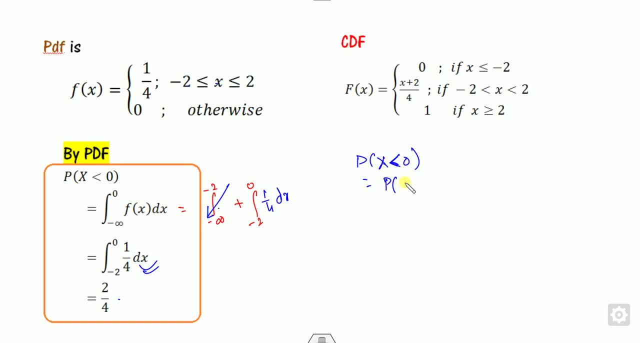 to required is in equality. So since it is already a continuous, so you can write it as here. So what is that? this is nothing but my f of 0. So where 0 lies, that 0 lies in this domain. So what? the answer is 2 by 4.. So look at, this method is always preferable because there 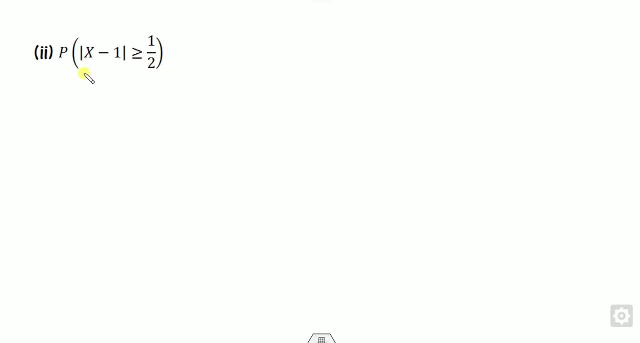 is no integration in that case, And similarly for this. now, since it's a modulus sign, so you firstly simplify it, I can write as 1 minus. Now it's a modulus sign, so you can write as a minus a to plus a, Then find the value of x. Now I can apply. this is the pdf rule. So 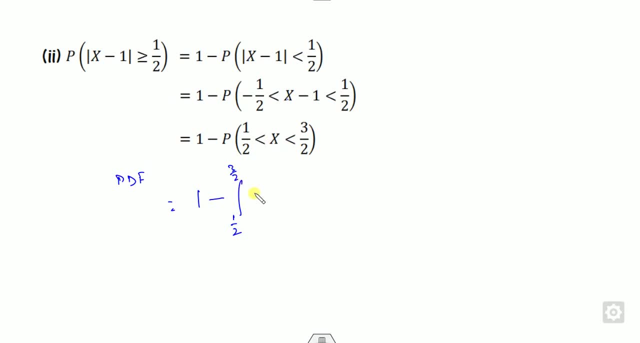 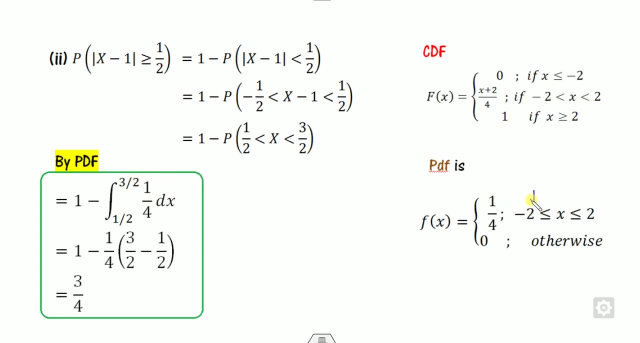 how you find this as 1 by 2 to 3 by 2, fx and dx. okay, and check whether 1 by 2 and 3 by 2 lies in the PDF. 0.5 and 1.5 lies in both them, so you can. 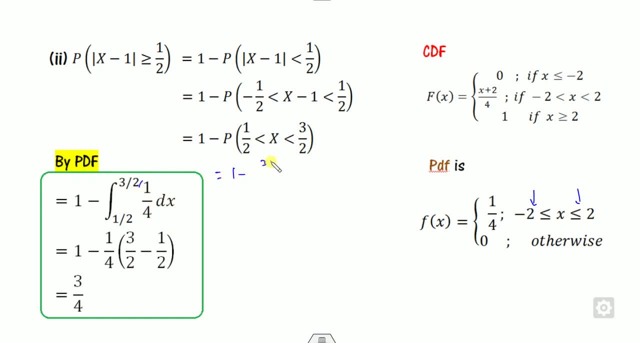 substitute the value of fx, as here. so look at that. this is nothing but my here. so what is the value of the fx when x lies between 1 by 2? 3 by 2 is nothing but 1 by 4. on the other hand, if you write: 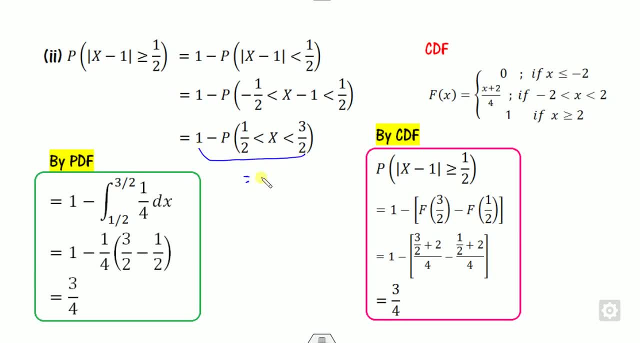 in the cdf form so you can write this term in the cdf. so how you write this as cdf is f of upper minus f of lower. okay, look at that. so what is f of 3 by 2? where is a 3 by 2 lies? 3 by 2 lies in. 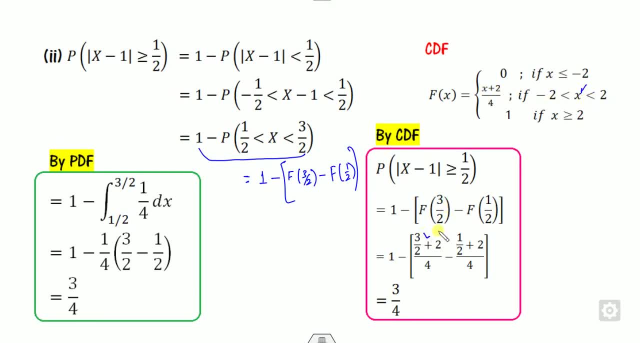 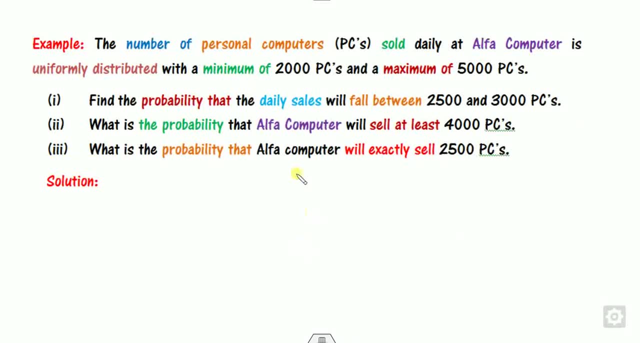 this interval, so it's 3 by 2 plus 2 divided by 4 and 1 by 2- lies also in this case. so look at that. answer simplifies: both are same. look at that. next example is a number of the personal computers sold. 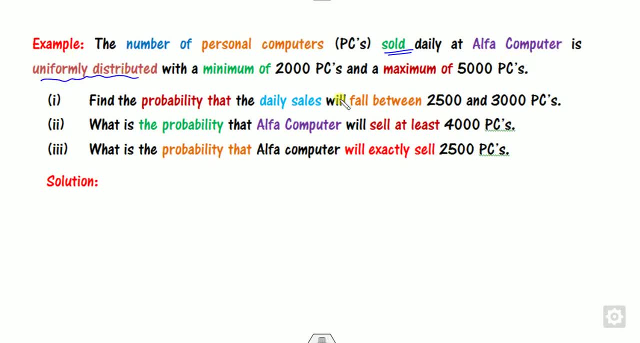 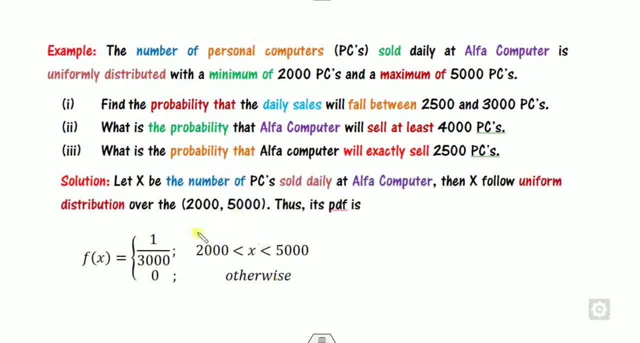 at the alpha computer is uniformly distributed, given that with the minimum is 1, 2000 and maximum is 5000. so what is the meaning is that this is interval is given 2000 to 5000 and it is a uniformly distributed. so you can define the pdf as 1 upon b minus a. 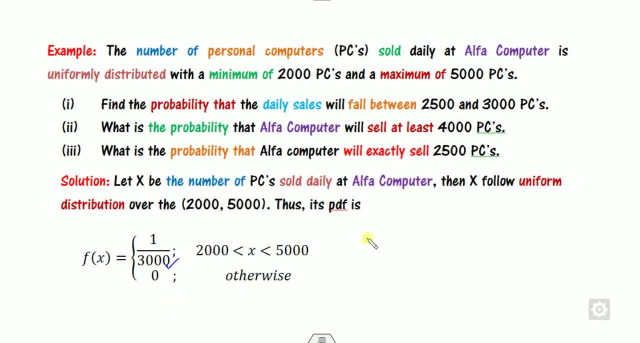 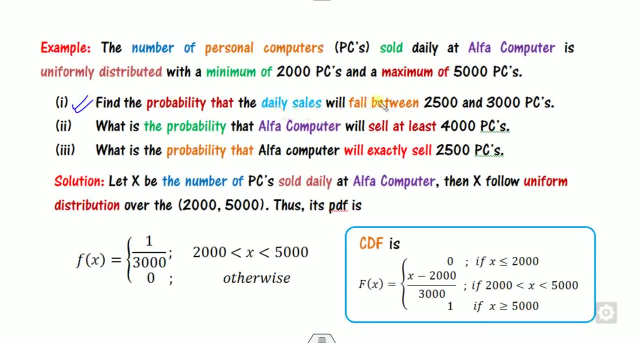 okay. so 5000 minus 2000 is 3000. also, you can define the cdf, okay. so first value is 0, next is x minus a divided by the range, and 1. so look at that, this is the cdf. now, what is the first task is that you have to find the value in between the 2500 to 3000. so this: 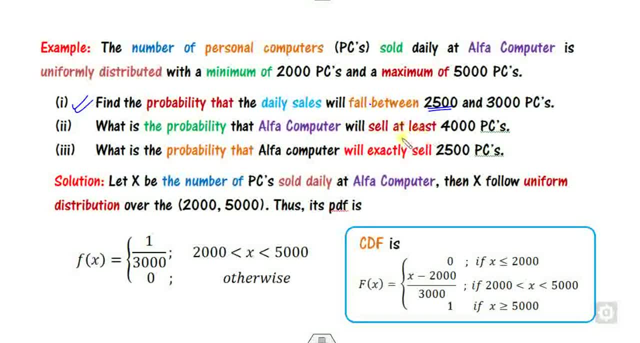 is the task you have to find. what is the second task? is you have to find at least four thousand. so at least four thousand means at least four thousand and exactly twenty five hundred. so these are the questions that we have to perform. so, again, we will solve each one with the help of the pdf and the cdf board. so firstly, you have to find it with the help of uh pdf. so you have to find it with the help of the pdf and the cdf board. so firstly, you have to find it with the help of pdf & see it here. here you can see, we have to find the absolute value as pi by 2 plus 0. 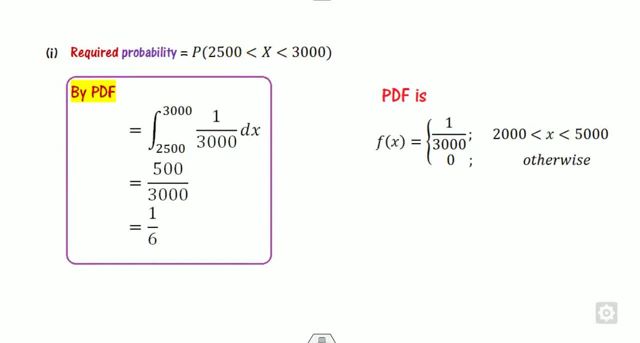 & 0, so we give k, which is one half plus k when you write pay less •. second can also say also times per is a simple rating, p with n as n as n, whatever situation, & p which one you want to pdf, so you have to define in in terms of the interval. this is my pdf. check whether this. 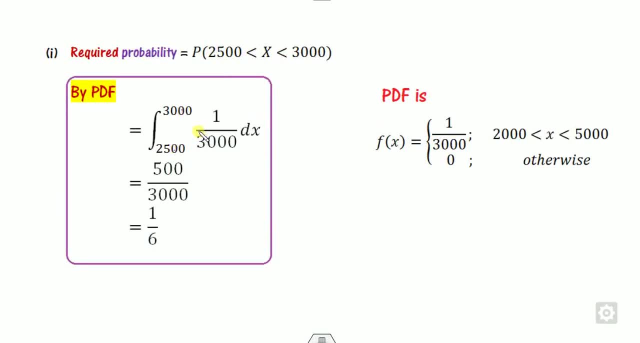 domain. both value lies in this interval. yes, so i can substitute. firstly, you can write it as like this way: this is 3000 f of x, dx. so what is the value of the fx in in this domain is 1 by 3000. so after simplify, this is 3000 minus 2500. you will get 1 by 6. on the other hand, if you write: 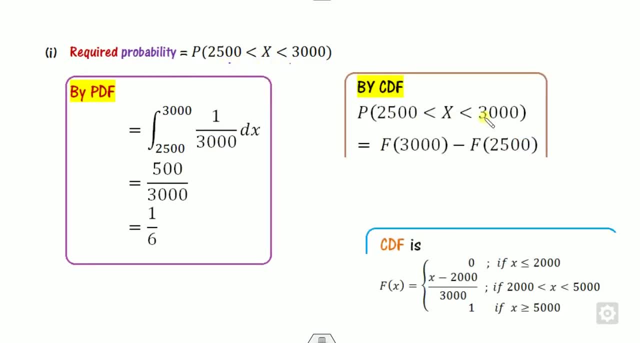 in the cdf form. so how you write that this is nothing but f of upper minus f of lower. so what is the f of 3000? so 3000 lies in the cdf. look at that. this is kept left. so 3000 lies here. so this: 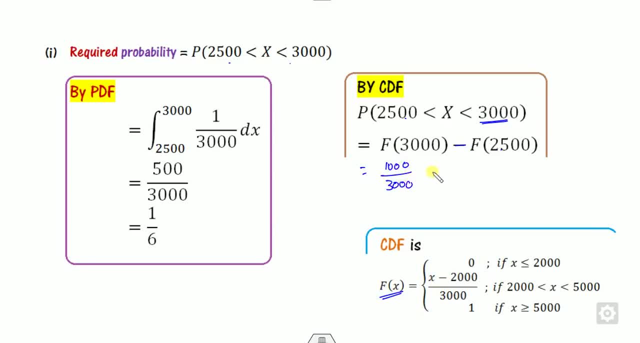 value is nothing but my 1000 by 3000. 2500 again lies here. so 25 minus 2000, 500 divided by 3000. so how you simplify that you will get these numbers. you look at that. the answers are: remain same. 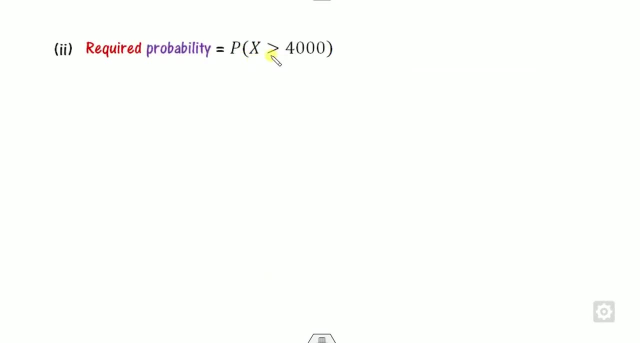 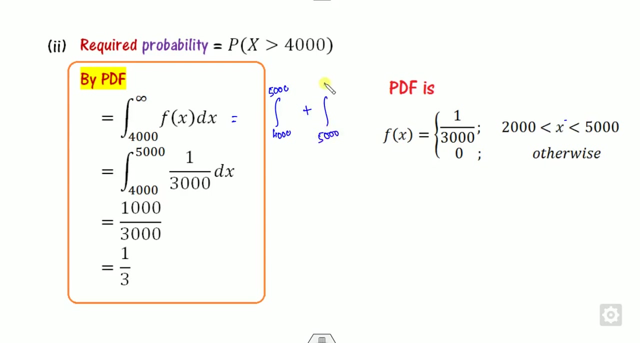 now second part is: at least the 4000 are there, so you will get solve this problem. so if you solve this with the help of the pdf, so how you solve that. this is 4000 to infinity fx of dx. so look at that, what is? the pdf is here so you can break this interval into 4000 to 5000 and 5000 to 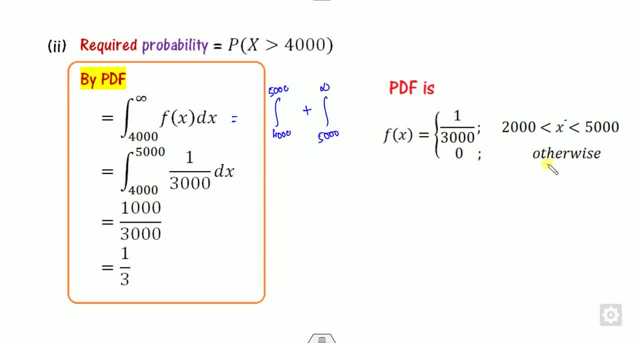 infinity. and what's the value of the 5000 to infinity of fx? look at that. otherwise is 0. so this is 0 and this is my 1 by 3000. so after simplify you will get 1 by 3. on the other hand, 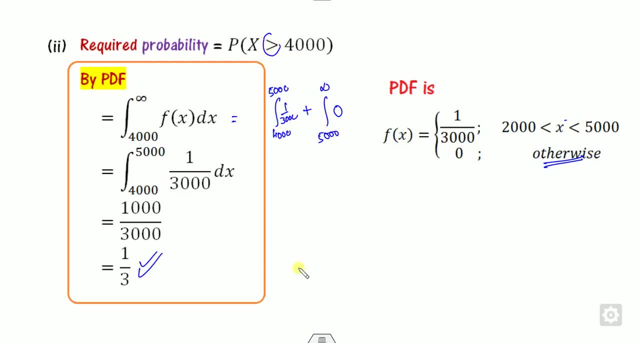 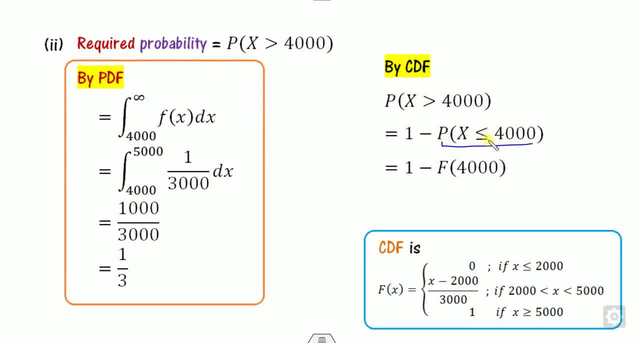 if you write in terms of the cdf, so you always wants to be a less than sign, so firstly, you can write as a 1 minus. so if you write as 1 minus, now look at that- what is that? it's a less than an equality sign. so this is f, this is a cdf, okay. so what is the cdf of 4000? where it lies that? 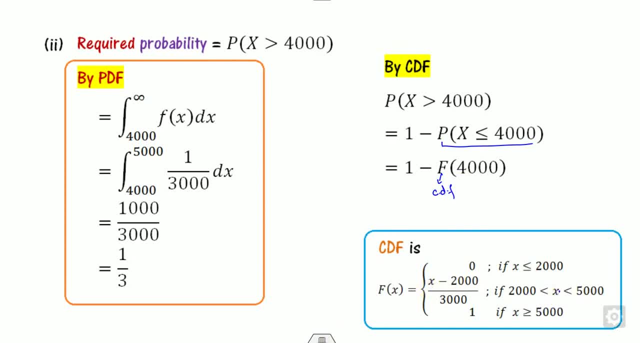 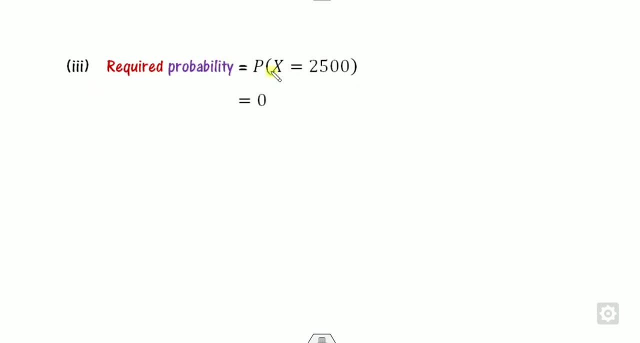 it lies here. so now 4000 minus 2000 divided by this, so you will get same answer again. what is the probability? that is, this is exactly 2500, so the answer is 0 always. why? because we have seen that whenever the x is a continuous, 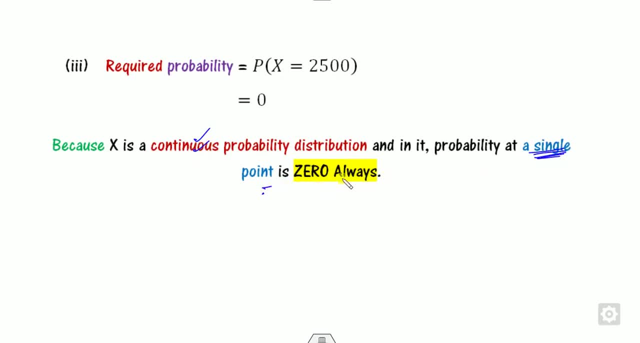 variable probability at a single point is always be a 0. okay, or you can also write like this way: it can be right. like this way: okay, because it's equality, so i can write like this way. okay, because it's equality, so i can write like this way. okay, because it's equality, so i can write. 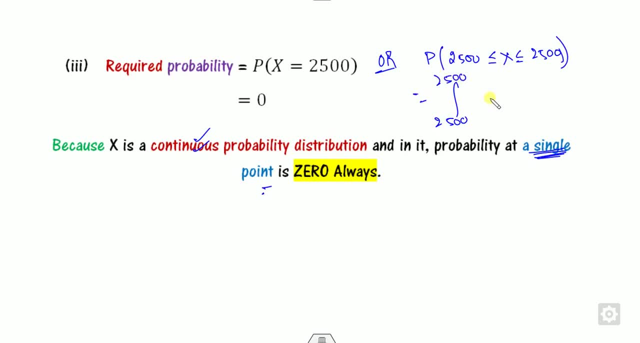 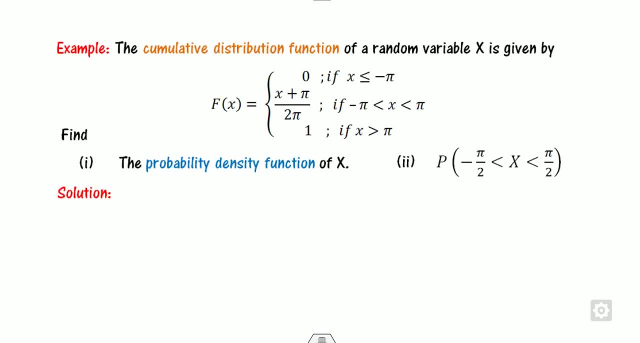 it here. So if you write in the integration form, so what will happen if the lower and upper limits are same? So the answer will always be achieved. Okay, look at one more example is here Now. in this case, this is a CDF cumulative distribution function- that 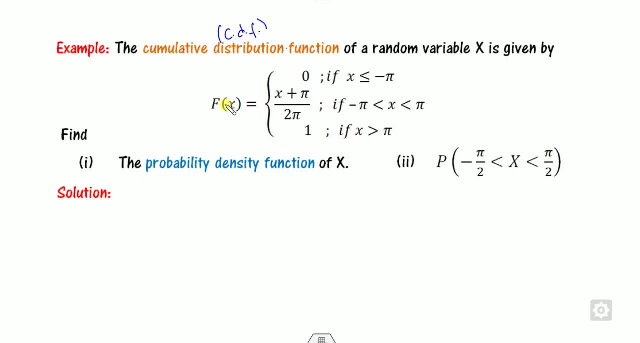 is a CDF is given to you that is a capital F and you have to find the PDF and you have to find this. So if I just try to find this, firstly by using the CDF, how you write that this is CDF of pi by 2 minus of minus pi by 2.. Okay, so what is the F of pi by 2, pi by? 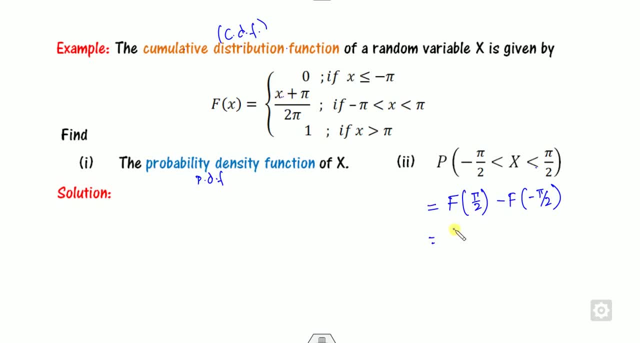 2 lies here, So x. you can substitute the value of x here. So it is my 3 pi by 2 divided by 2 pi. If it is x is minus pi by 2, it's my pi by 2 divided by 2 pi. So what is that this? 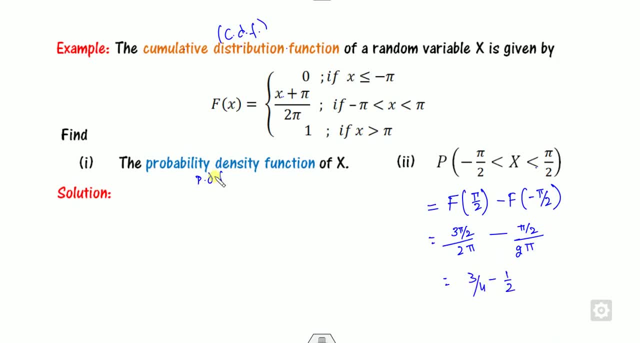 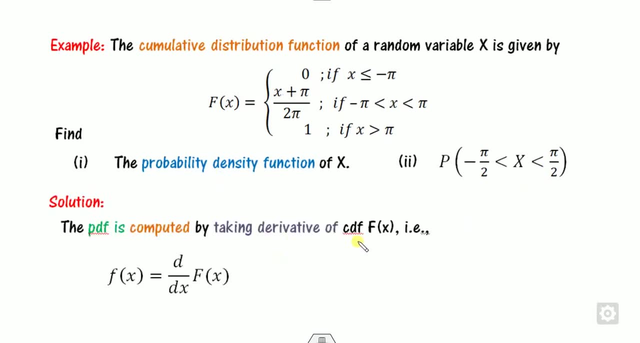 is my 3 by 4 and this is 1 by 4 is required, But how you find the PDF. So remember that whenever the CDF is given and you want to find the PDF, you always get the derivative of the CDF. So f of x is here. So what is? 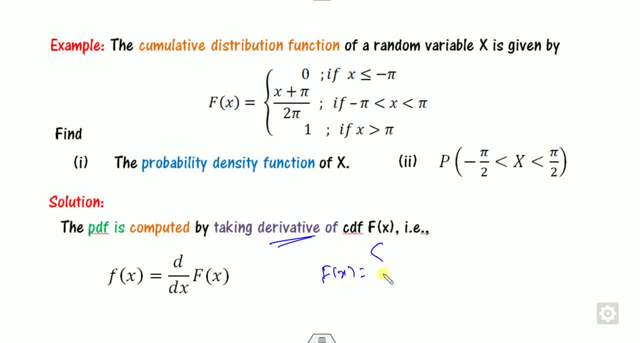 the derivative of this. How you find that Okay. so what is the derivative of first part is 0.. What is the derivative of the second part is 1 by 2 pi 1 is again 0. So 0 is already. 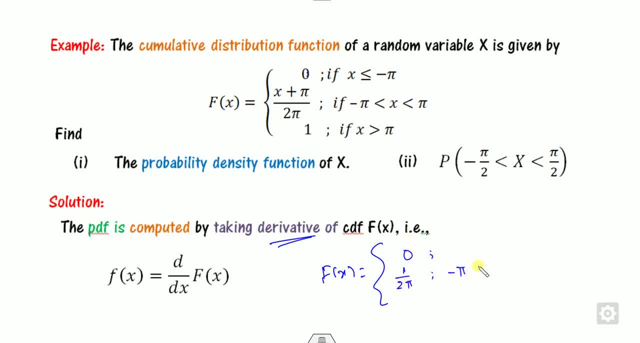 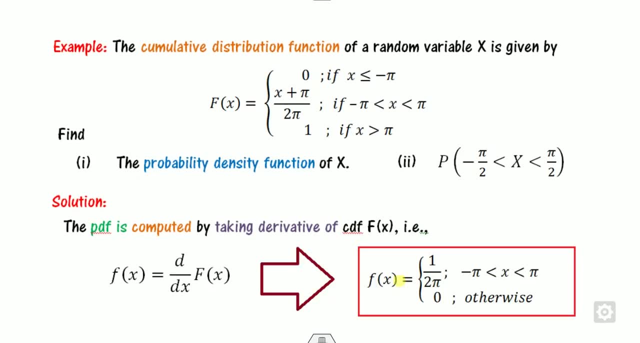 written. So value of this is a constant quantity and it lies in the domain this and otherwise we can say that 0.. So this is my small fx And this is my PDF. Now you can solve this problem with the help of either PDF or CDF. 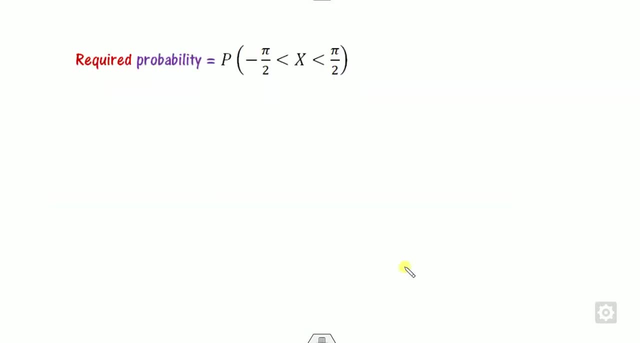 both Okay, so you can prefer any one of them. So let's do with a both way. So if I use this as a PDF, so I can write: firstly, minus infinity to the plus pi by 2, minus pi by 2 to plus, 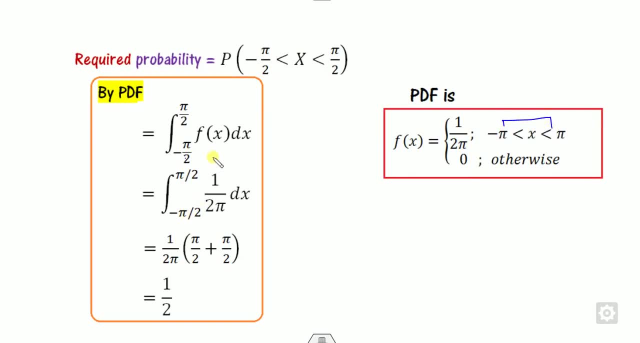 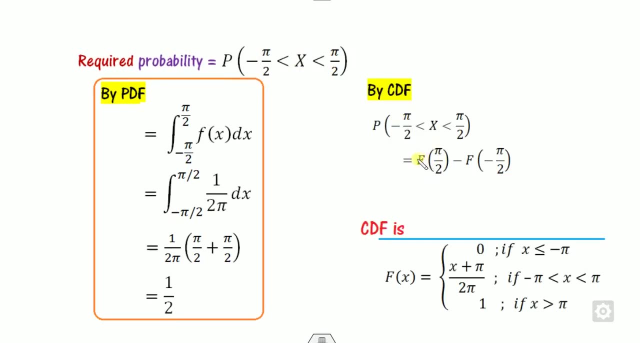 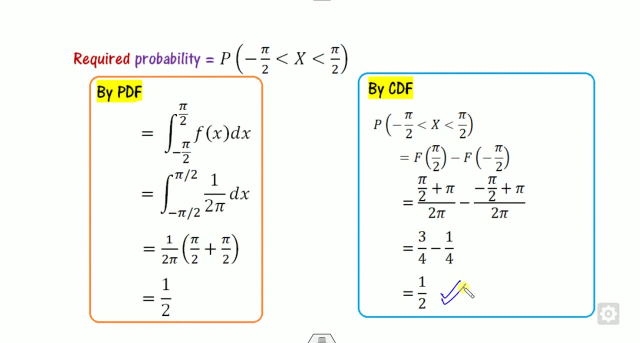 pi by 2 and both lies in this interval, So you can write the value of the fx as here. So after solving, you will get this. On the other hand, if you want to write this in the CDF, This so pi by 2 lies here, So you can substitute this value, this you will get as a this answer. 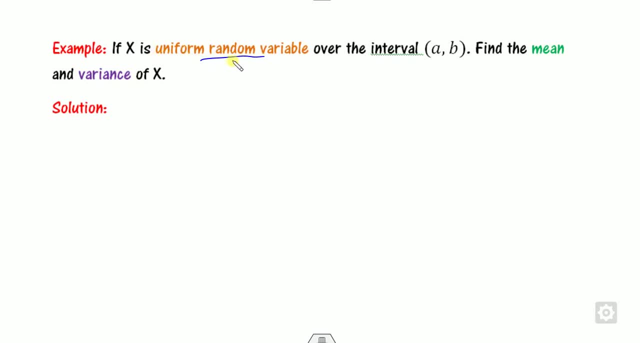 Look at the last example. is there? Suppose x is a uniform distribution, random variable over the interval a- b, Then you have to find what is the mean and the variance. For example, we have seen that in the binomial distribution what is the mean is np, Variance is npq. Similarly, 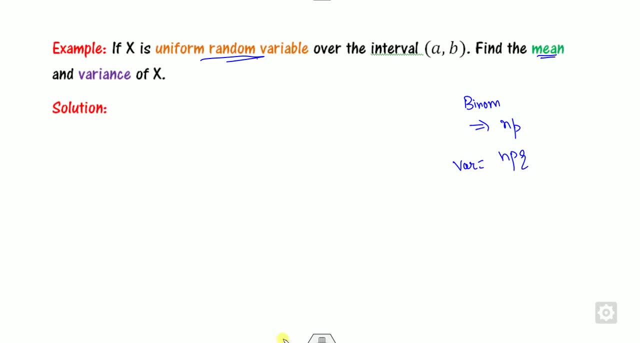 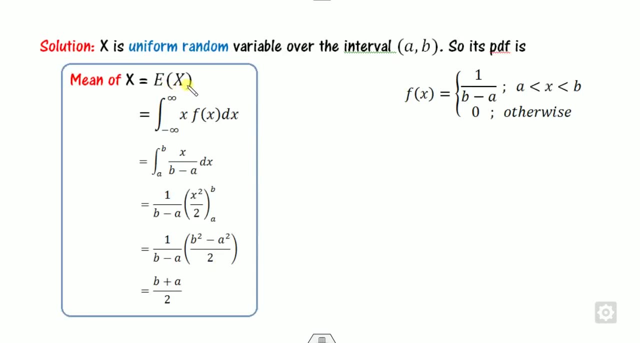 you have to find the mean and the variance of uniform distribution. So what is that? is this format? You have to find it as 0 here. So one more time, this pdf is given to you how you find the mean is v of x. What is the formula for the mean is x into f of x. So 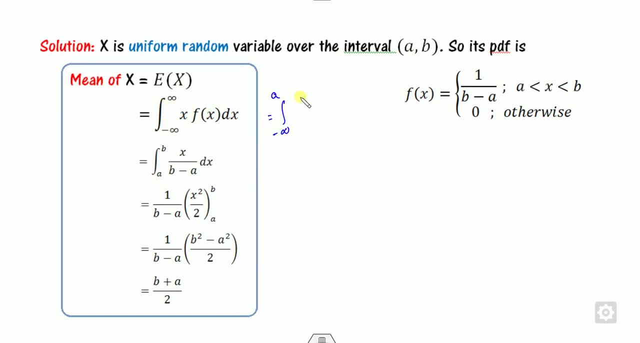 this: minus infinity to infinity. you can break from minus infinity to a, then a to b and then b to infinity. The value of this is 0. value of this is 0. only a to b is here, So now you can integrate them. So 1 upon b minus a is outside integration of x, is x squared by 2.. 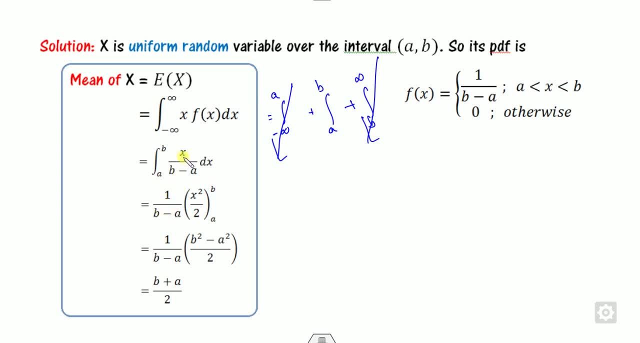 So after solving, you will get this pdf is given to you. For this, you need to send a pdf to the Grandpa. actually, in case I have to participate, this- Okay, now you need to come back and do the same thing- is to take the energy which you have in this even- And I will beOne- energize. 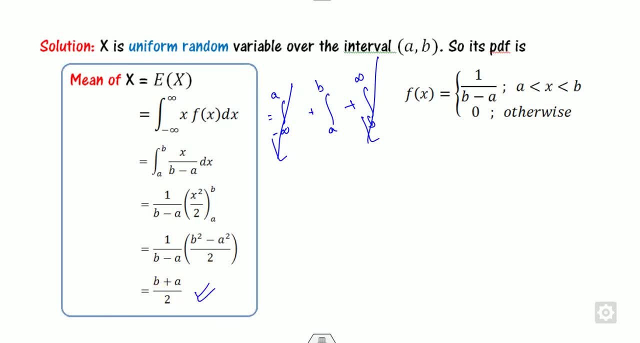 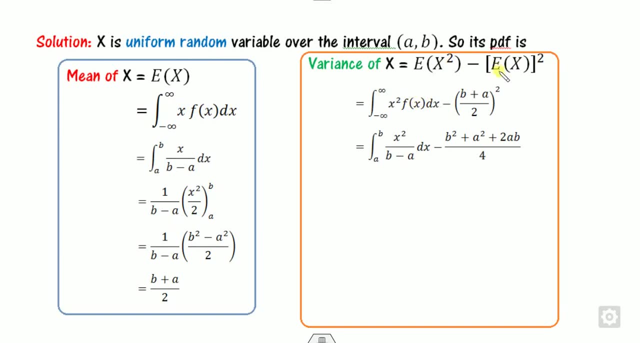 you will get b plus a by 2.. Similarly, you can find the variance. What is the variance? is e x square minus e x whole square. So what is the e x square? is x square into f x? This is nothing but my mean, So we have already calculated the mean as this. So how? 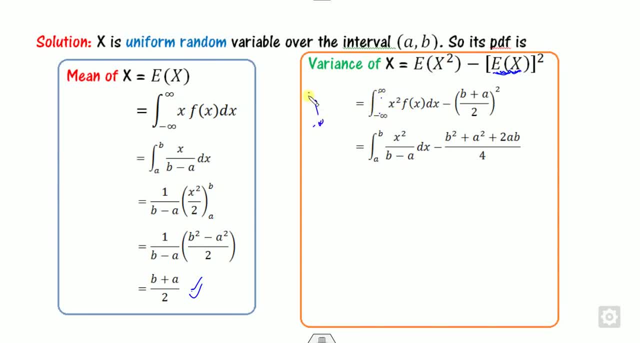 you solve this Again, you have to decompose this into the three portion, this a to b and then b to infinity. So first and last are 0 here, And now again 1 upon b minus a is outside. Integration of the x square is x cube, And this is there. So simplify this. 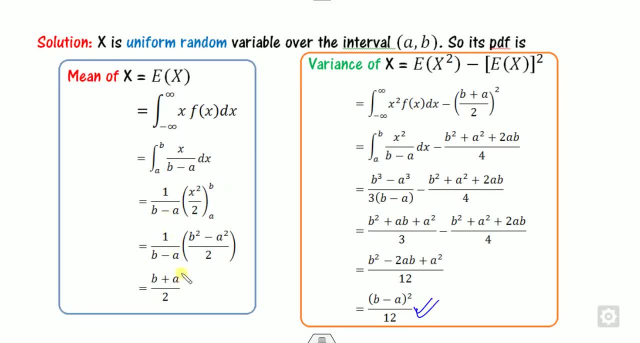 You will get. this is required So you always remember that mean is nothing but b plus a by 2.. That is the average of this, While the variance is b minus a square by 12.. So look at one example corresponding to mean and variance so that it will be clear to you. Suppose x: 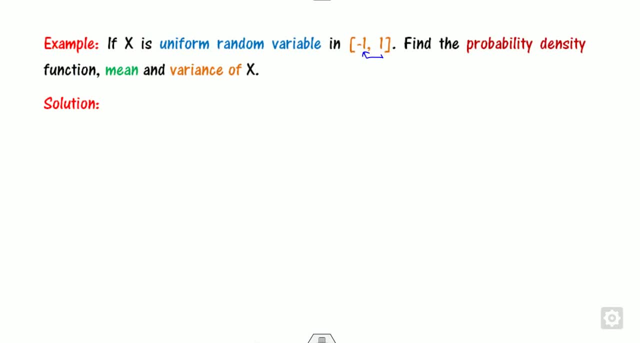 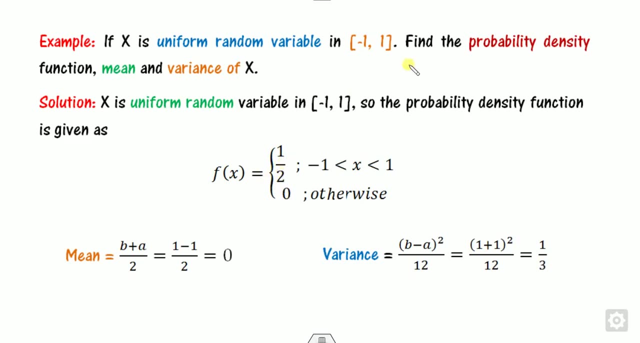 is a uniform random variable lies in the interval this. So firstly you have to define this pdf. So 1 upon b minus a. So b minus a is 1 plus 1, 2. So this is the pdf. So this is the first part. answer You. 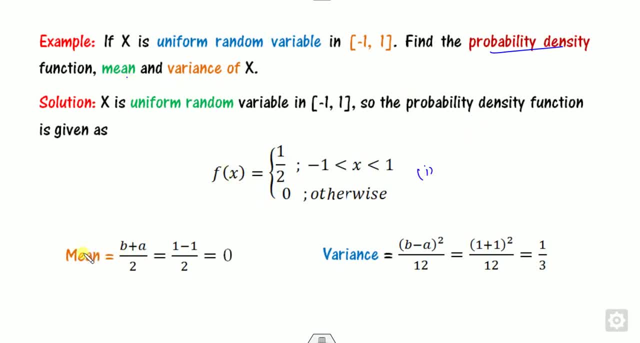 have to find the mean. So there is no need to calculate it, because we know that the mean of the uniform distribution is a plus b by 2.. So this is b, this is a, So it's a: 0, and the variance is my b minus a whole square by 12.. So we will substitute here, You will. 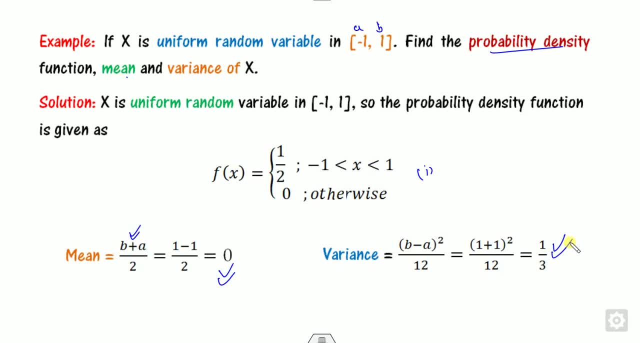 get 1 by 3.. So this is a simple procedure that you can solve the any uniform distribution problem with the help of the pdf. Now we will learn the master clever. Now, if there is a problem, if there is no problem, how to solve it. So I will write mark here, blank a and. 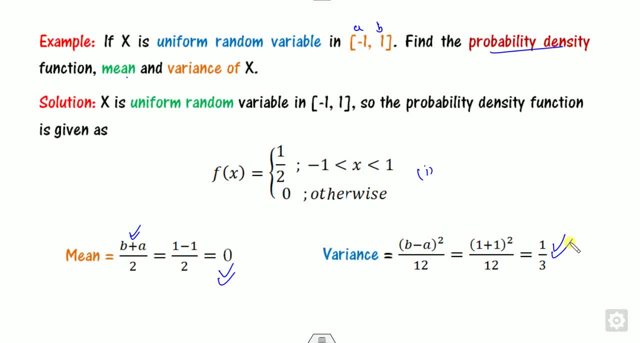 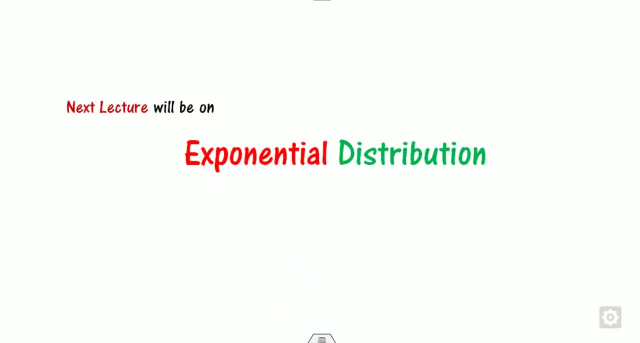 this is because count 1 and you have to find the bulk you can use to calculate the spoke. So pdf and the cdf both. so i always prefer the cdf because it is takes less time. so we will see in the next lecture that the exponential distribution. if still there is any doubt, you can contact me.